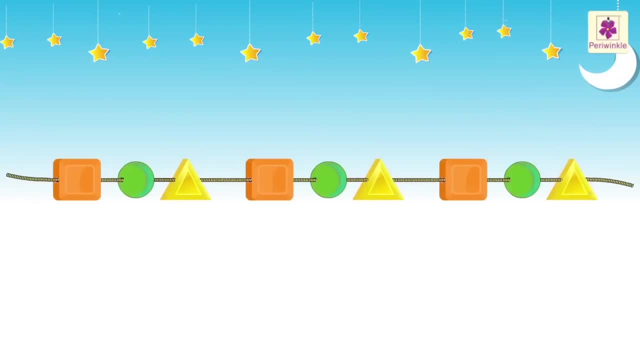 Look at the bracelet. We have a square, circle, triangle, Square circle, triangle, Square circle, triangle, Circle triangle, and so on. This is called a pattern, as it is repeating itself. Look, we got the pattern. 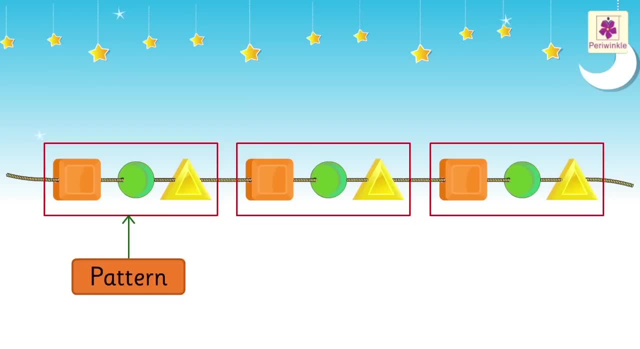 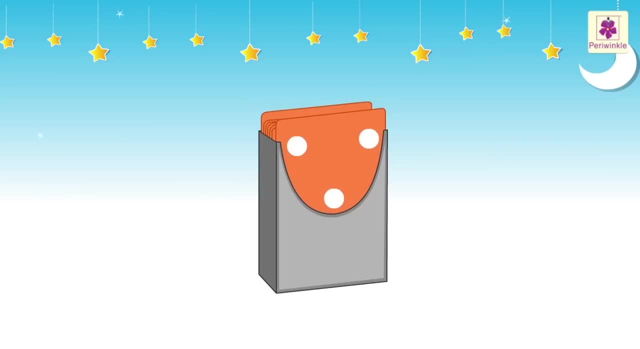 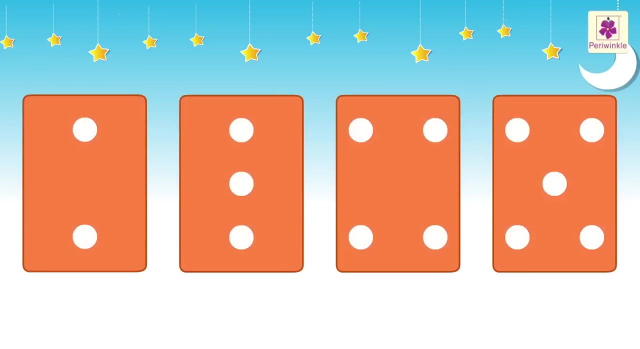 Now let us try making few more patterns. Look at this pack of flashcards. Each card has a pattern of dots. Look, we have arranged few cards according to the increasing order of the dots, Starting with a card with two dots, three dots, four dots, five dots. 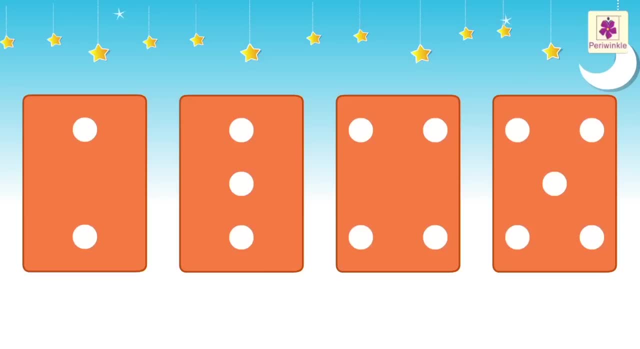 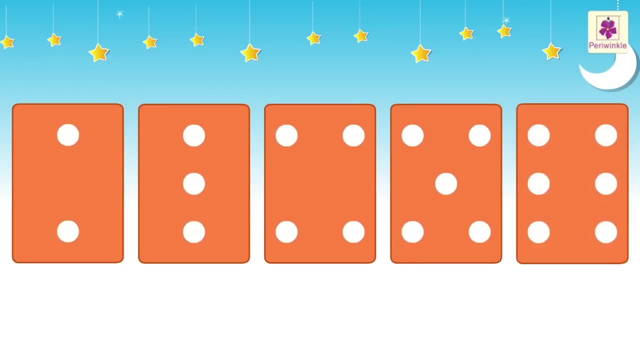 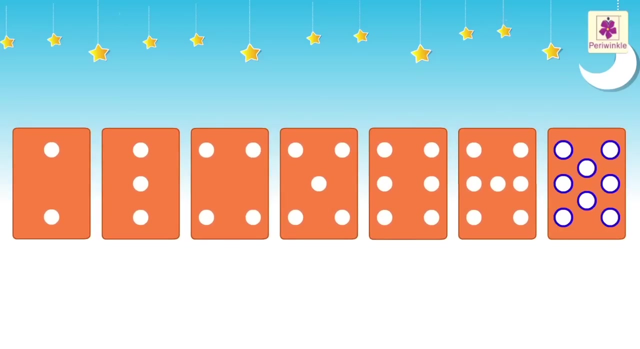 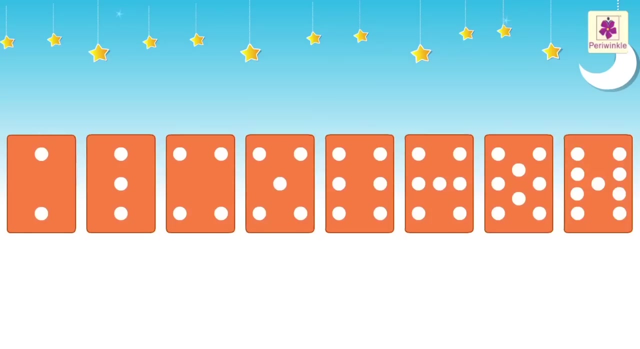 Kids. let us follow the same pattern and find out the next four cards. Yes, correct, The next card, The next card will be with six dots, then seven dots, then eight dots and lastly nine dots. Kids, isn't it interesting. 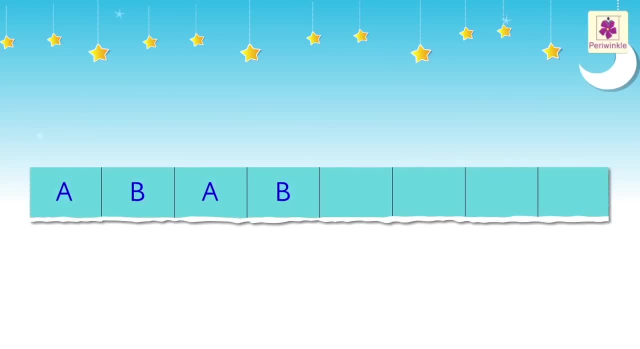 We can find pattern in letters too. Now observe the given pattern and write the next four letters. We can see that letter A and letter B are the same. Letter A and letter B are placed alternatively. This becomes our pattern, So the next letter will be letter A, then letter B. 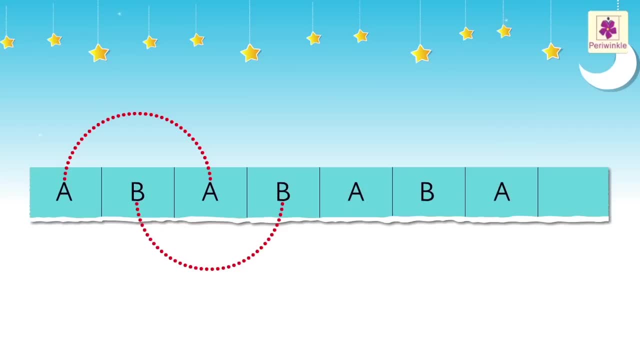 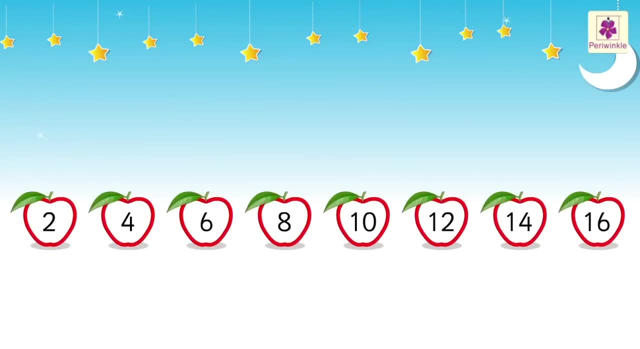 Then again letter A and lastly letter B. Did you know we find patterns in numbers also? Let's see how, Starting with numbers Number 2, When we skip count by 2's, we get 4, 6, 8, 10.